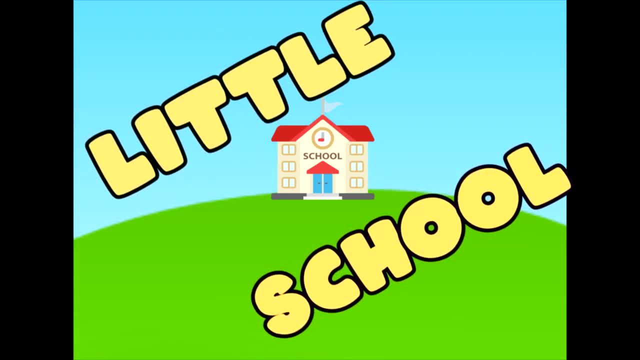 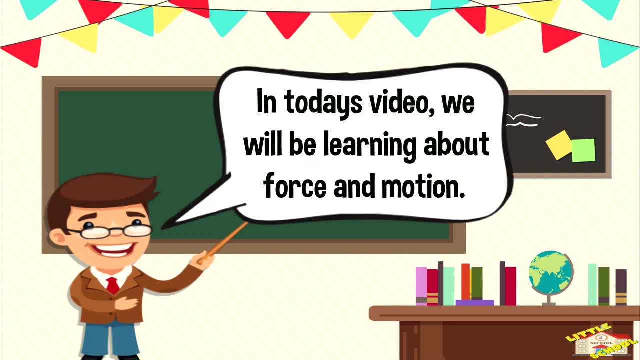 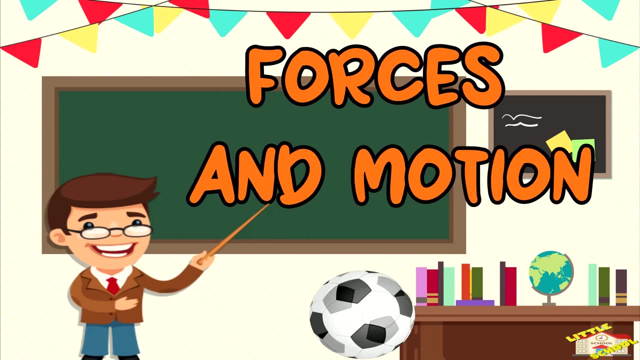 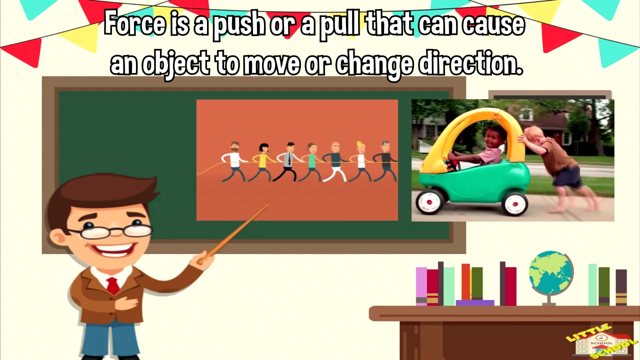 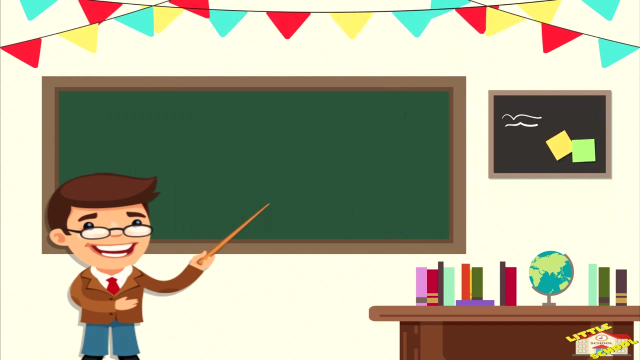 Hey kids, In today's video we will be learning about force and motion. Are you ready? Let's begin. What is force? Force is a push or a pull that can cause an object to move or change direction. Here's an example of force: Opening and closing a door. You apply force to twist the doorknob. 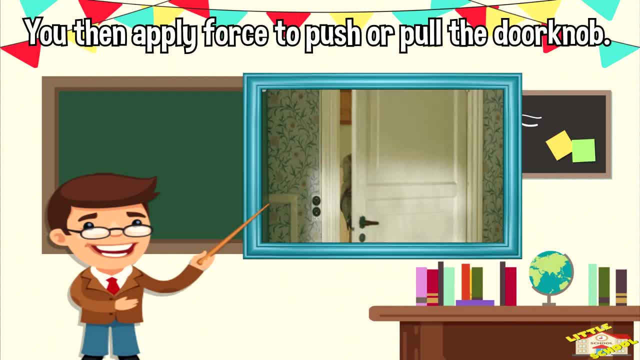 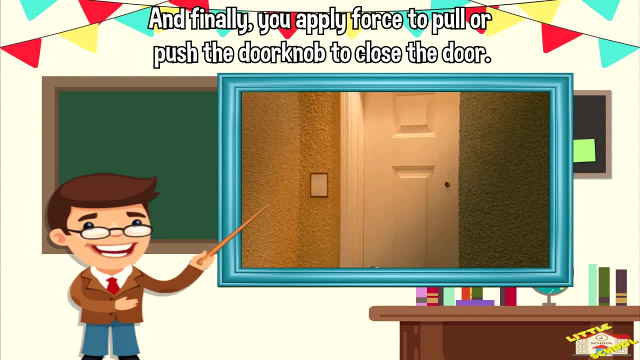 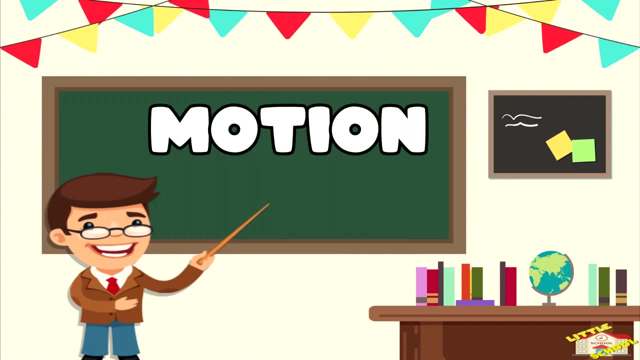 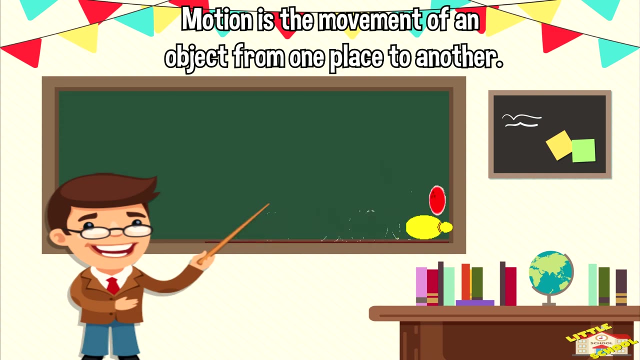 You then apply force to pull the doorknob And finally, you apply force to pull or push the doorknob to close the door. What is motion? Motion is the movement of an object from one place to another. Here's an example of motion. 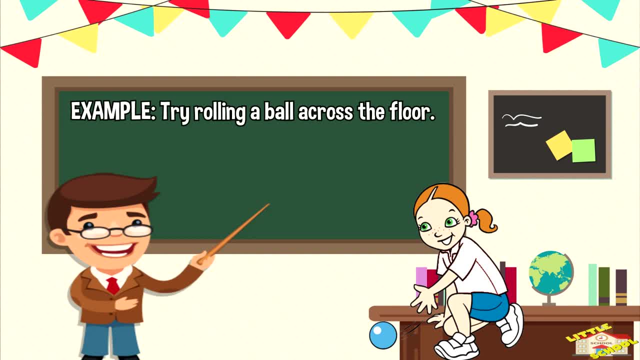 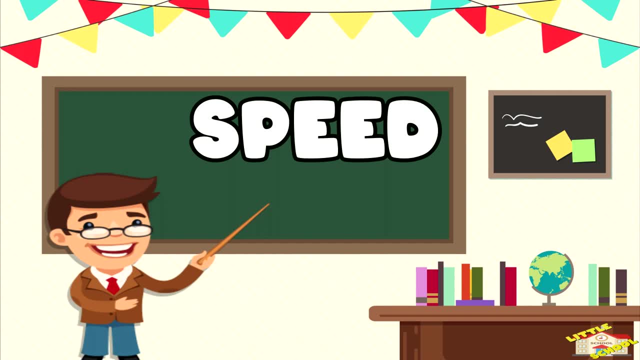 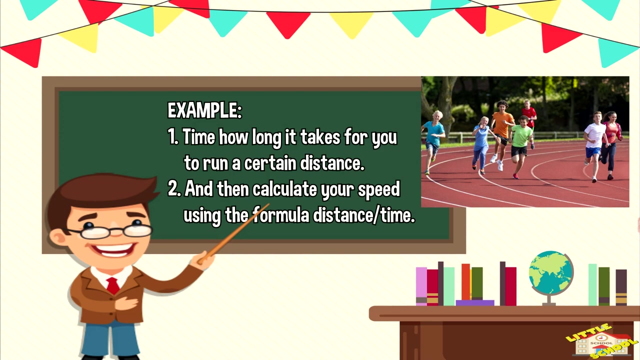 Try rolling a ball across the floor and observe how it moves. What is speed? Speed is how fast an object is moving. Here's an example of speed Time: how long it takes for you to run a certain distance And then calculate your speed using 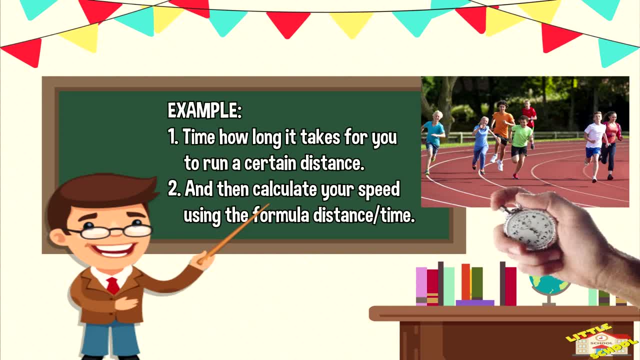 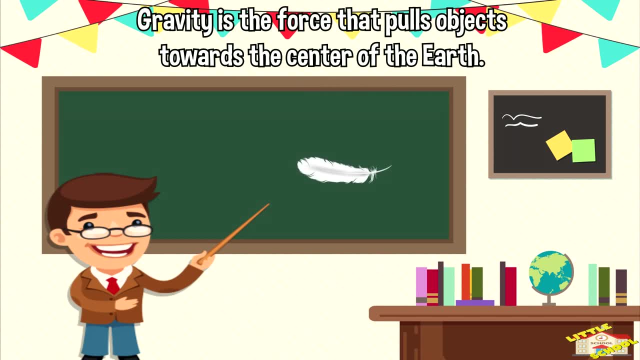 the formula distance divided by time. What is gravity? Gravity is the force that pulls objects towards the center of the earth. Here's a great example as to how to observe gravity: Try dropping objects of different weights from a height and observe how they fall. 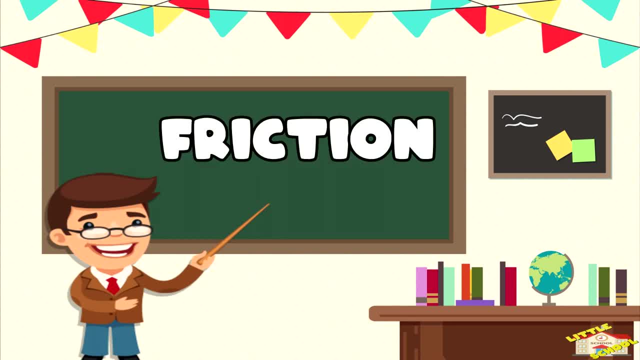 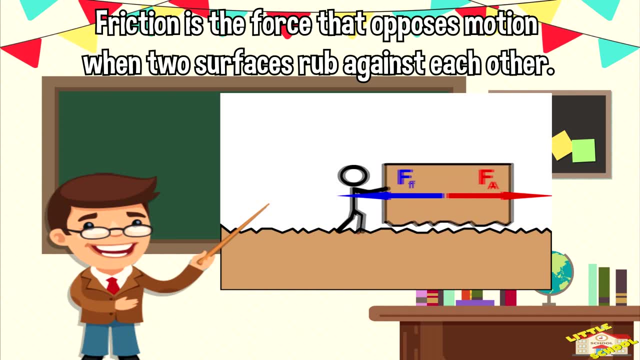 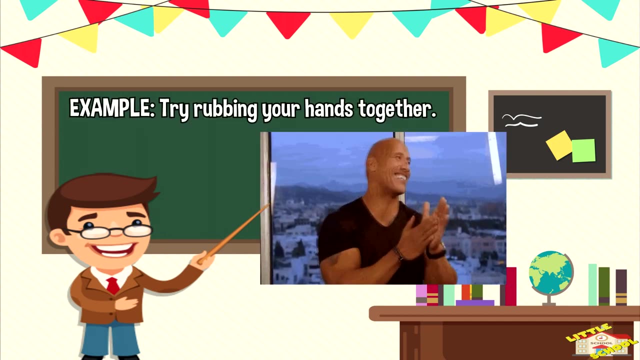 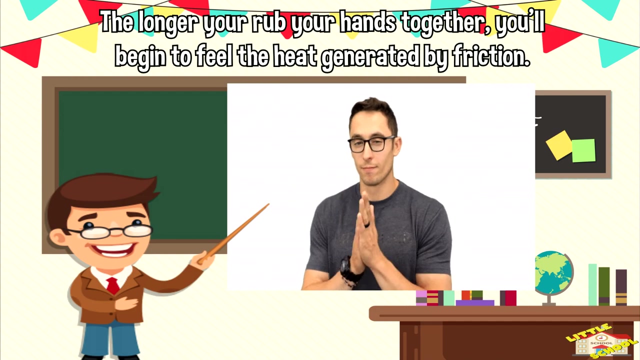 What is friction? Friction is the force that opposes motion when two surfaces rub against each other. Here's a great way to observe friction: Try rubbing your hands together. The longer you rub your hands together, you'll begin to feel a heat generated by friction. 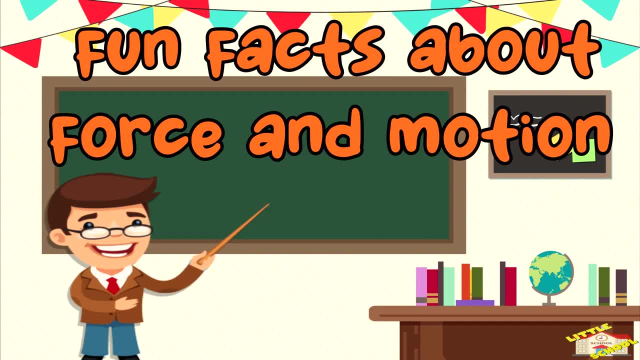 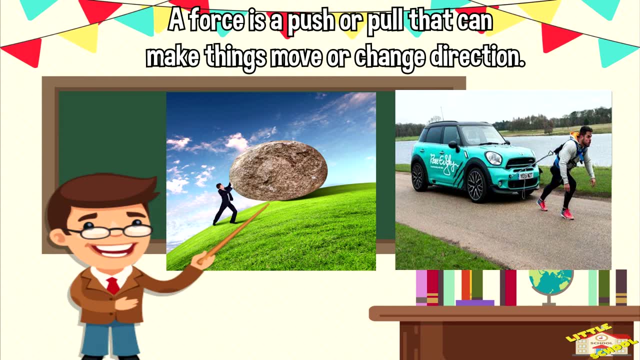 Now here are fun facts about force and motion. What is friction? Fati Wins and Gl mass Fati can look at an object at any time and Beispielical Yourung can look at a head looking at an object and a head looking at an object. 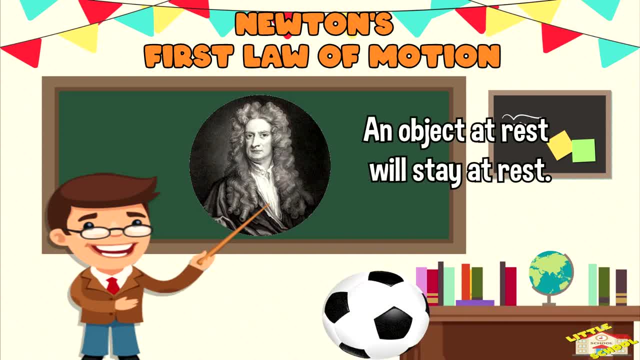 A force is a pulling force. Now let's see what this can do. Fati can do: push or pull things or move or change direction. Force causes objects to slow down, speed up or change shape. A force is a push or pull that can make things move or change direction. A force can also cause objects to slow down, speed up or change shape. 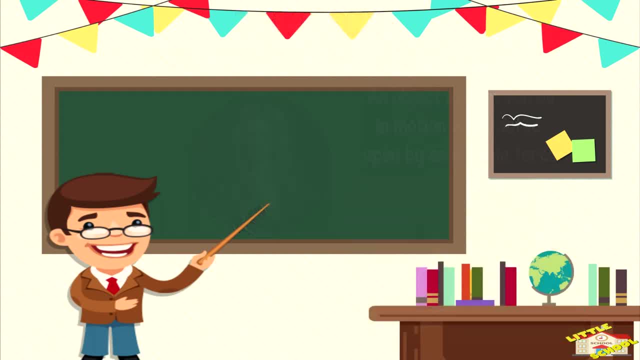 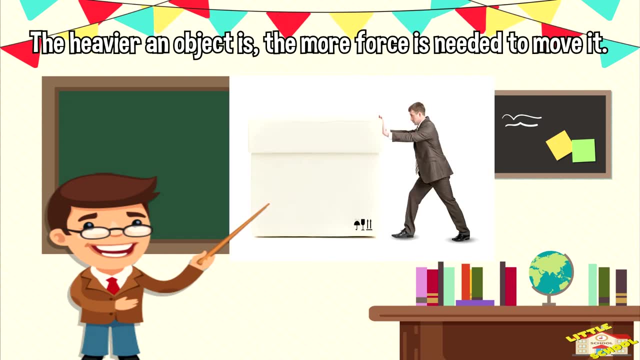 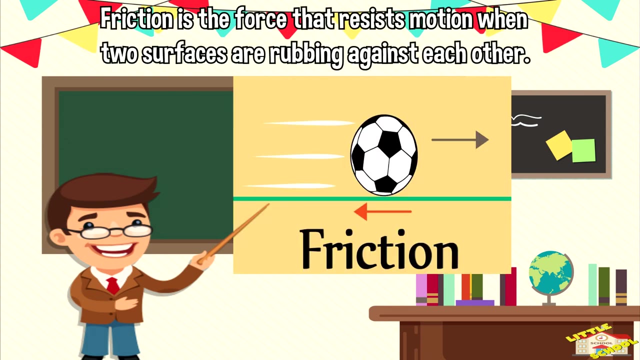 acted upon by an outside force. The amount of force needed to move an object depends on the object's mass. The heavier an object is, the more force is needed to move it. Friction is the force that resists motion when two surfaces are rubbing against each. 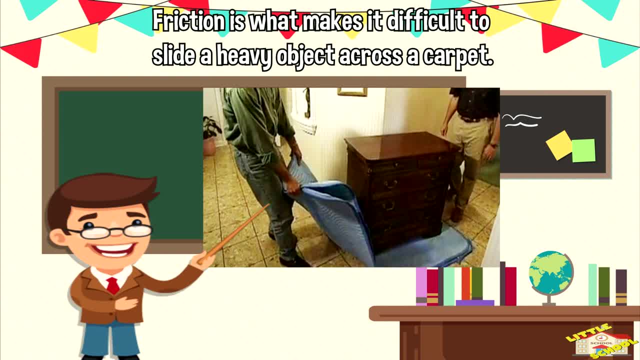 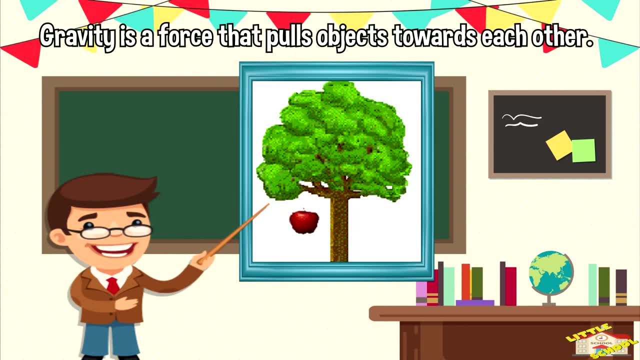 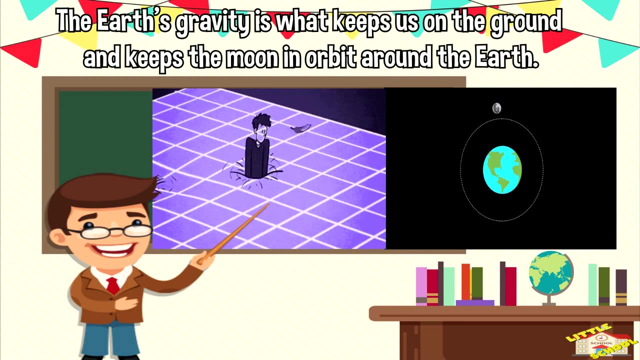 other. For example, friction is what makes it difficult to slide a heavy object across the carpet. Gravity is a force that pulls objects towards each other. The Earth's gravity is what keeps us on the ground and keeps the moon in orbit around the Earth. 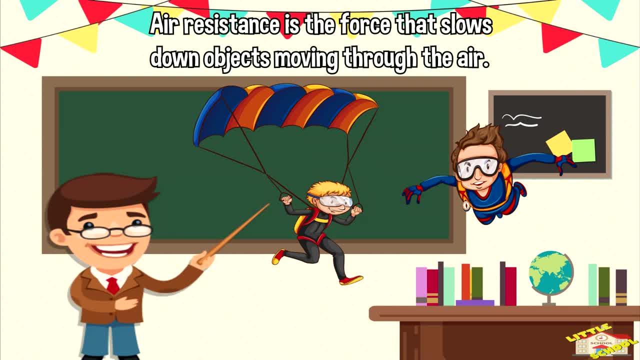 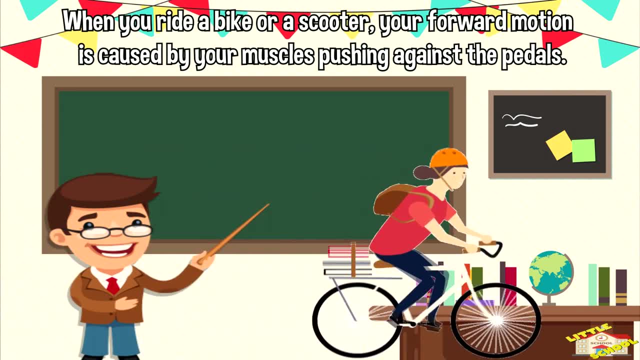 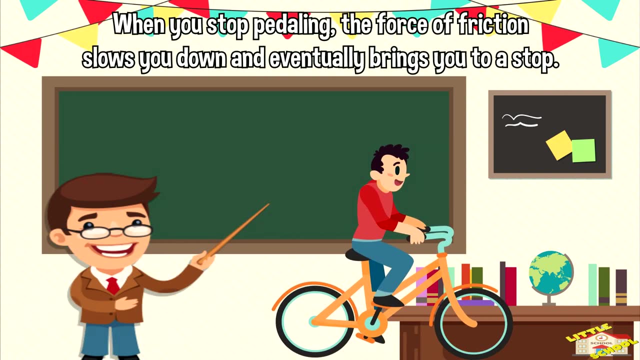 Air resistance is the force that slows down objects moving through the air, such as parachute or a skydiver. When you ride a bike or a scooter, your forward motion is caused by your muscles pushing against the pedals. When you stop pedaling, the force of friction slows you down and eventually breaks your 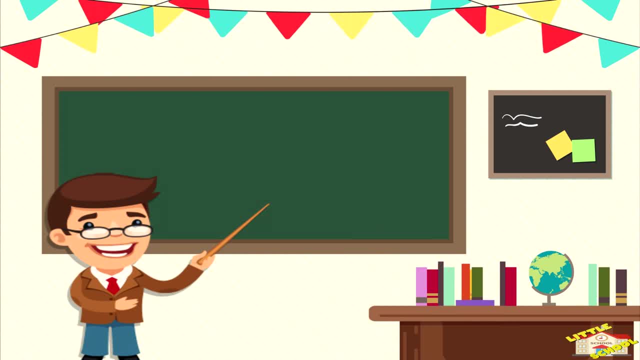 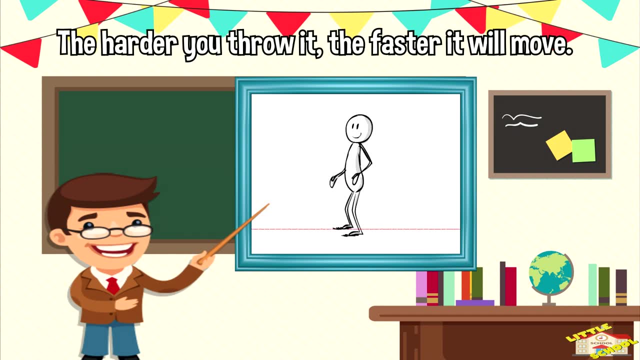 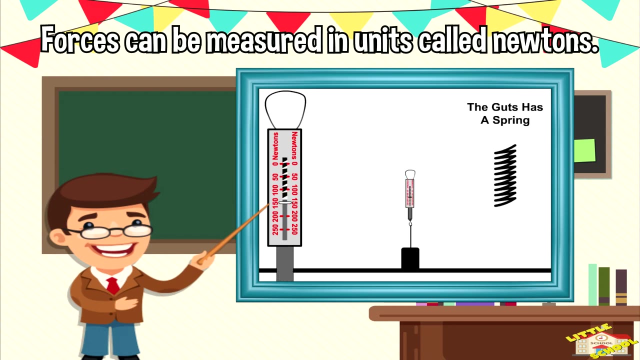 balance. This brings you to a stop. When you throw a ball, you are using a force to make it move. The harder you throw it, the faster it will move. Forces can be measured in units called Newtons. The stronger the force, the more Newtons it has. 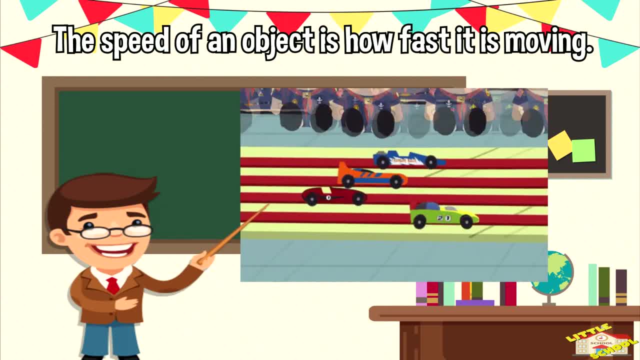 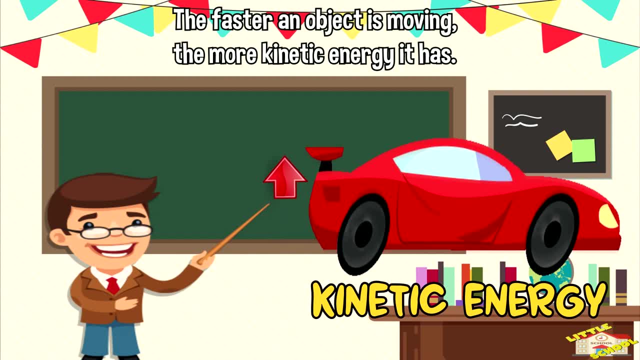 The speed of an object is how fast it is moving. The speed of an object is how fast it is moving. The speed of an object is how fast it is moving. The faster an object is moving, the more kinetic energy it has. And that is all for today's video.